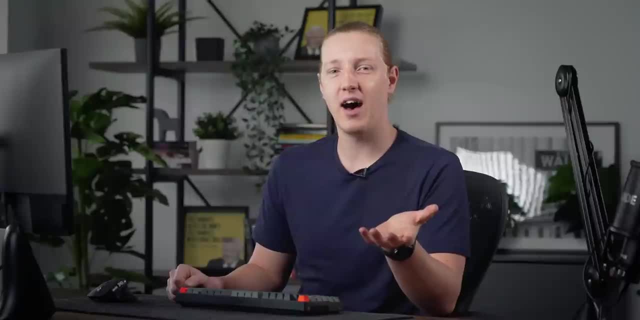 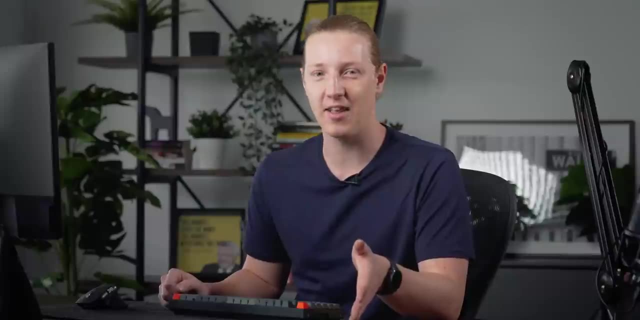 Have you guys ever asked your partner how they're feeling, only to be greeted with the classic I'm fine. What do you think when they say I'm fine? Usually it's a telltale sign that they actually aren't fine at all. In fact, usually it's quite the opposite. Well, 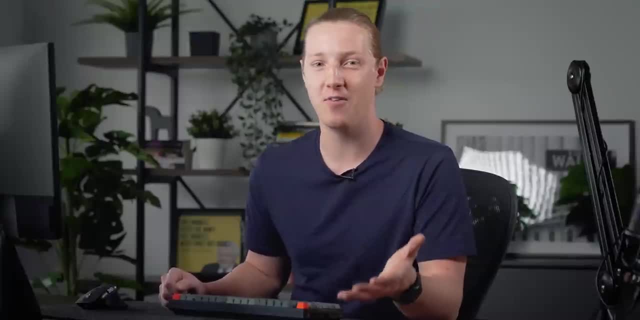 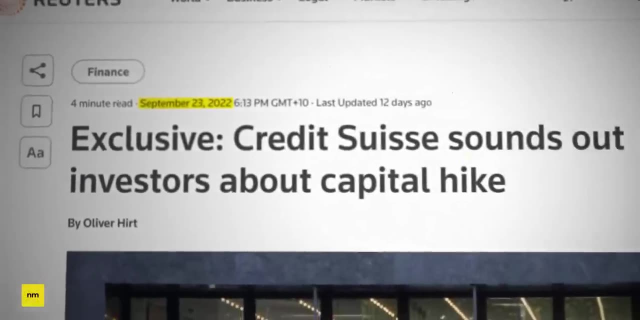 it turns out, Credit Suisse have just played the don't worry, I'm fine card, and you guessed it. it's now backfiring, So let's dive in. It all started a few weeks ago when reports emerged that Credit Suisse may look to do a capital raise. Now, investors haven't been. 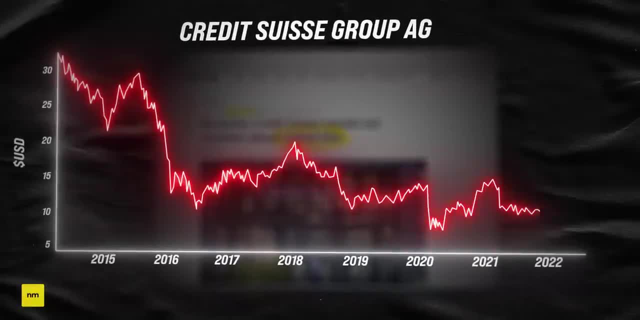 too happy with Credit Suisse. They're not happy with Credit Suisse. They're not happy with Credit Suisse. for a long time now, really, since 2015, the stock has just sucked, And it's no secret that they've definitely been caught up in some pretty bad scandals from. 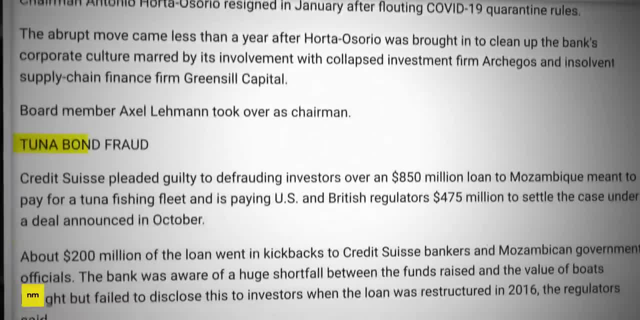 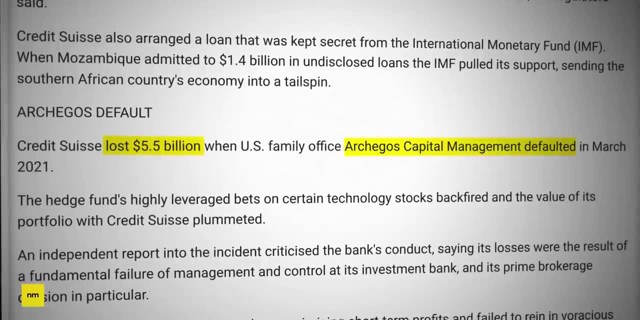 failing to stop money laundering by cocaine traffickers, to the tuna bond fraud, to the green seal scandal, to copping a whopping $5.5 billion loss through the RK Ghost default in March last year. Fair to say, management has been questionable at best, And with so. 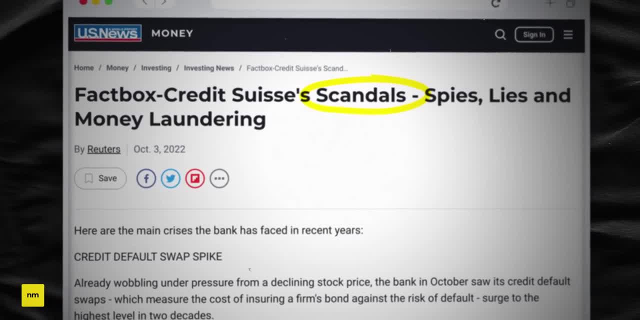 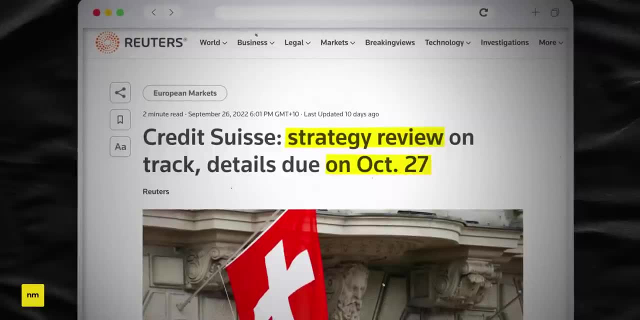 many blunders really hampering the company over the last few years. the firm is now set to straighten the record. Credit Suisse is the first company to announce a major restructuring of the business, on October 27th. Only problem is they might need a bit more money to make that happen, and since the 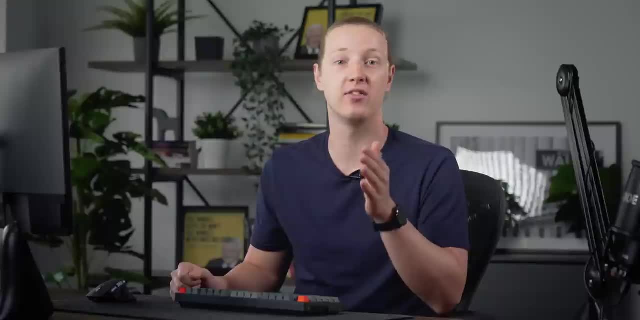 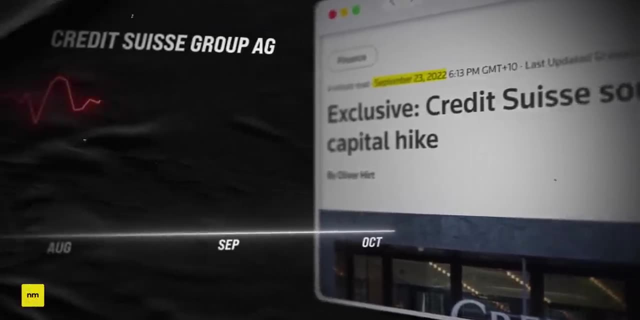 reports of a potential 4 billion Swiss franc capital raise hit the press a few weeks ago. the stock has really plummeted. Reuters first reported rumours of a capital raise on the 23rd of September, the same day that Credit Suisse stock shed 12.5%. They noted, quote: 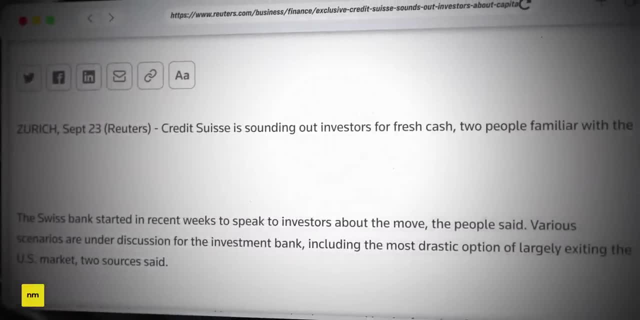 Credit Suisse is sounding out investors for fresh cash. two people familiar with the matter said Approaching them for the fourth time in around seven years. it's a determination that credit Suisse is going to be a big hit. Credit Suisse has been in the business for seven years as it attempts a radical overhaul. 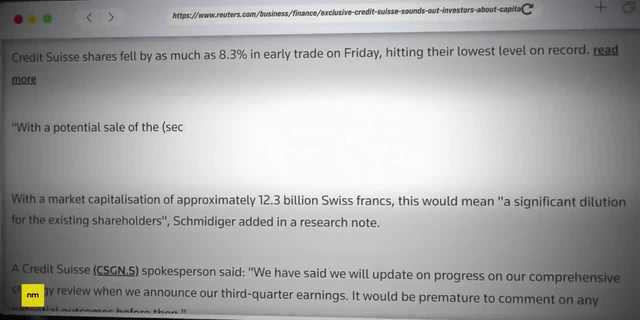 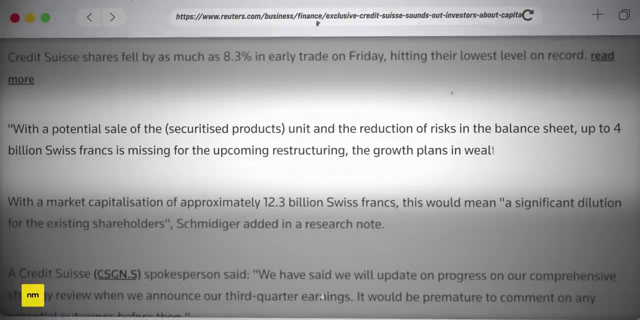 of its investment business Quote, with the potential sale of the securitised products unit and the reduction of risk in the balance sheet, up to 4 billion Swiss francs is missing for the upcoming restructuring, the growth plans in wealth management and for the accumulation. 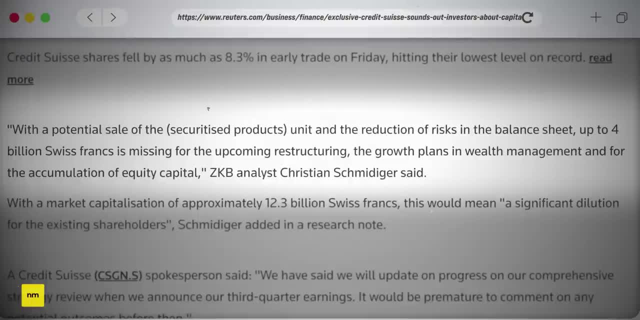 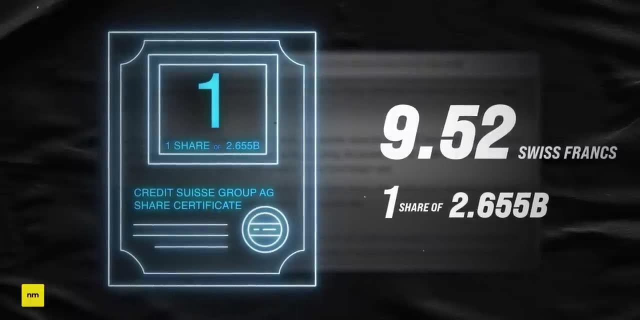 of equity capital, ZKB analyst Christian Schmidiger, said So sounds like they need money. but if they resort to raising capital after the stock has created 55% over the past 12 months, well that's painful for shareholders as, beyond the paper loss, they now get the added bonus of the stock. Credit Suisse is now in the business for the third time in around seven years as it attempts a radical overhaul of its investment business Quote, with the potential sale of the securitised products unit and the reduction of risk in the balance sheet up to 4 billion Swiss francs. 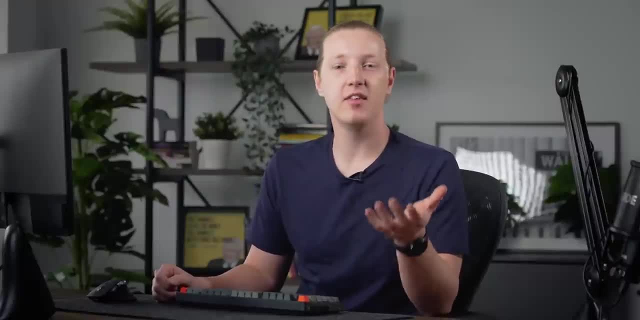 is missing for the upcoming restructuring, the growth plans in wealth management and for the accumulation of equity capital, ZKB analyst Christian Schmidiger said. But speaking of investor confidence, beyond the share price tanking, this news has also sent the prices of Credit Suisse credit default swaps soaring. 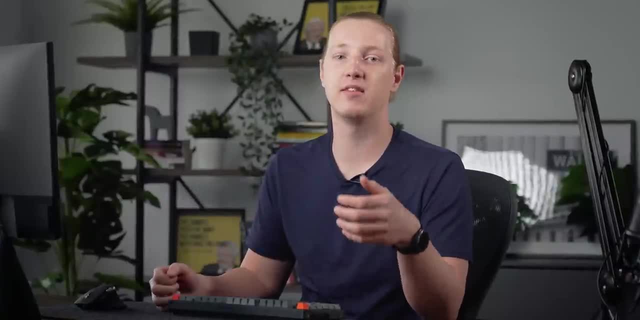 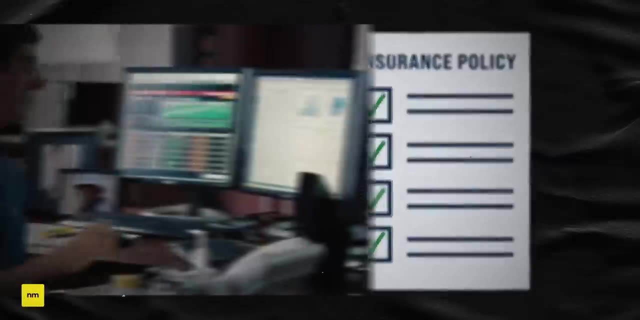 And this is where a lot of the 2008 financial crisis comments on Twitter are coming from. Now a credit default swap is similar to an insurance product And yes, they're what Michael Burry bought back in 2005 in anticipation of that financial crisis. 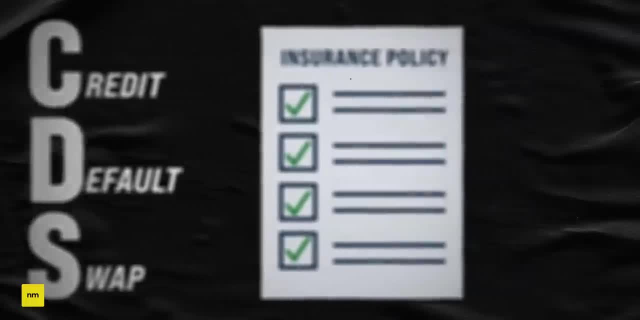 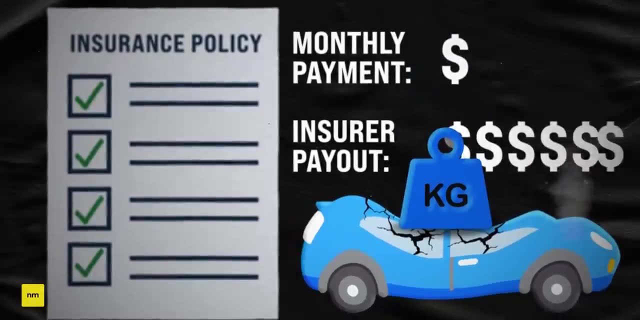 So to make sense of credit default swaps, just think about car insurance. You purchase an insurance policy to protect you against financial consequence if your car gets totaled. So it's the same thing with a credit default swap. In this particular case, we're buying. 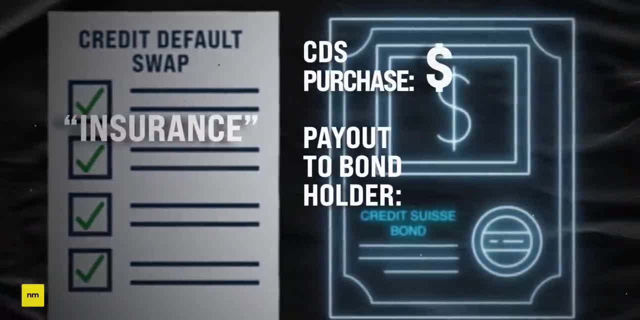 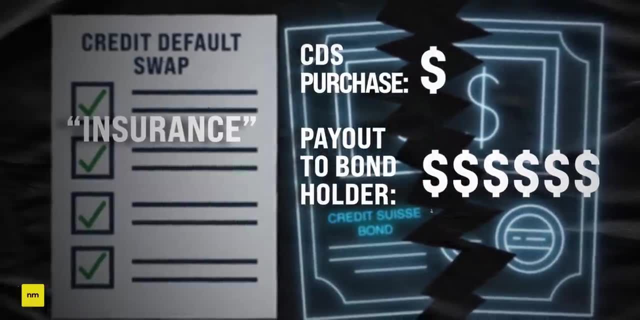 the credit default swap as protection against Credit Suisse's bonds defaulting and thus Credit Suisse not being able to pay us, the bond holder. Now, as you might expect, if the investors that hold these bonds are starting to worry about the stability of the bank, they might look to buy some of these swaps. Remember. 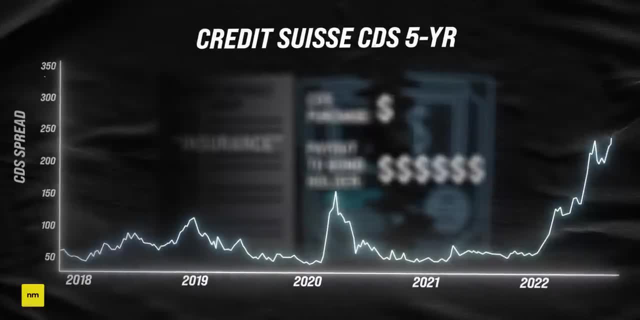 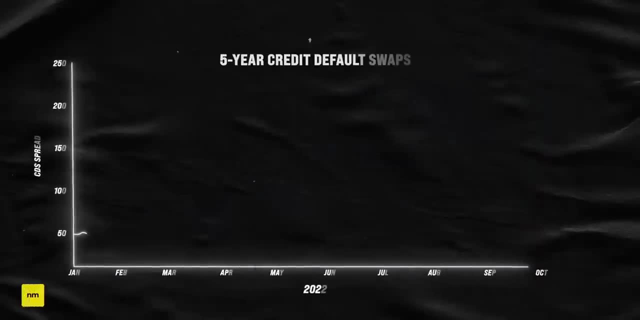 that would give them insurance in case Credit Suisse blows up. And, like any financial asset, when there's high demand and everyone is buying, that pushes up the price of the asset. Now have a look at what's happened in the credit default swap market. This is the price. 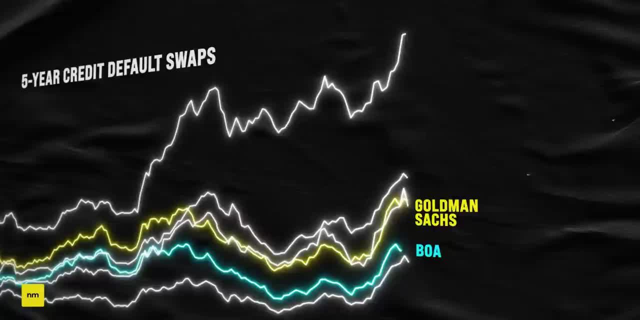 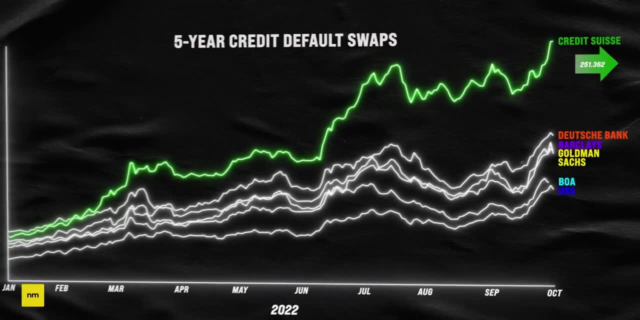 chart for the five year credit default swaps for Bank of America, Goldman Sachs, Barclays, Deutsche Bank, UBS and Credit Suisse. One of these is definitely not like the others. Investors are buying Credit Suisse credit default swaps hand over fist, And now they're. 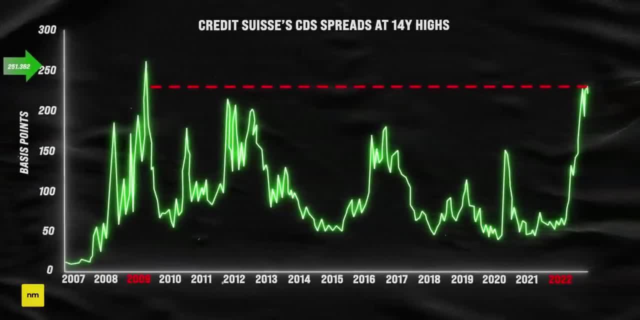 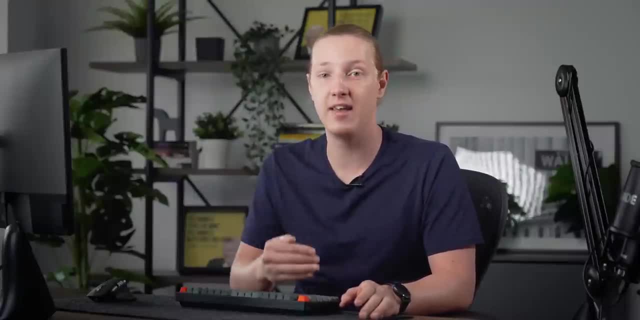 the same prices that they were in 2009.. It's pretty scary, But that in itself isn't an indicator of financial stress. Remember, that is just an indicator of investor sentiment. But this is definitely where Credit Suisse starts to shoot itself in the foot, And this 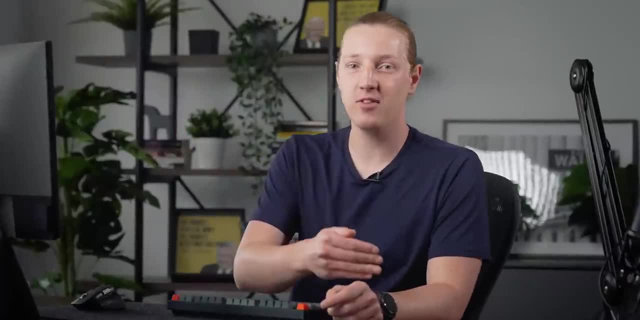 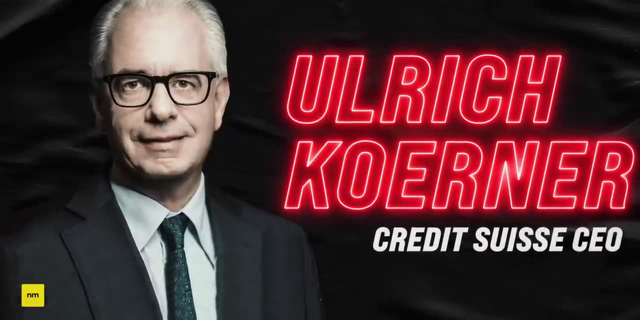 is the I'm fine honey moment because, in response to this poor investor sentiment, their CEO, Ulrich Körner, on Friday decided to send out an unprompted company wide memo to reassure staff investors that everything is going to be all right. He said, quote: 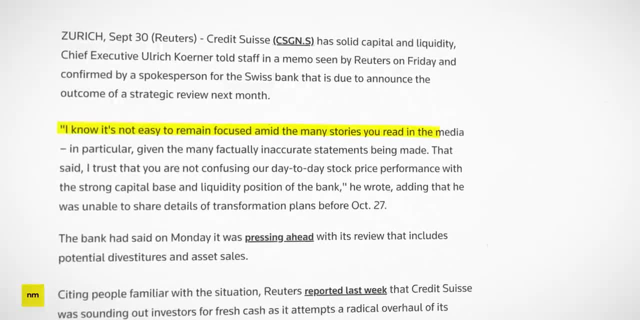 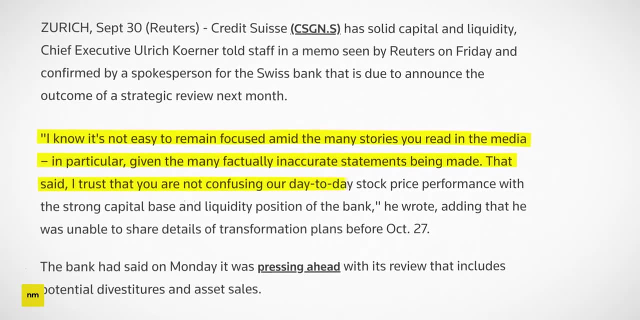 I know it's not easy to remain focused amid the many stories you read in the media, in particular given the many factually Inaccurate statements being made. That said, I trust you are not confusing our day to day stock price performance with the strong capital base and liquidity position of the bank. Hmm, 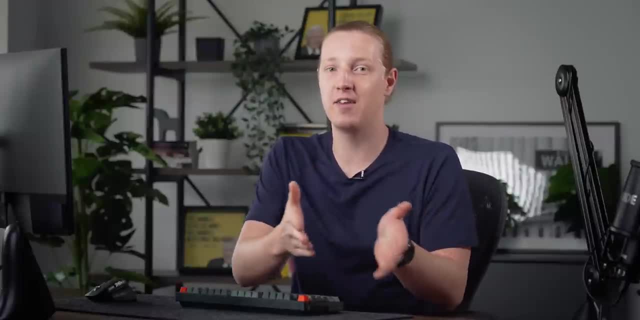 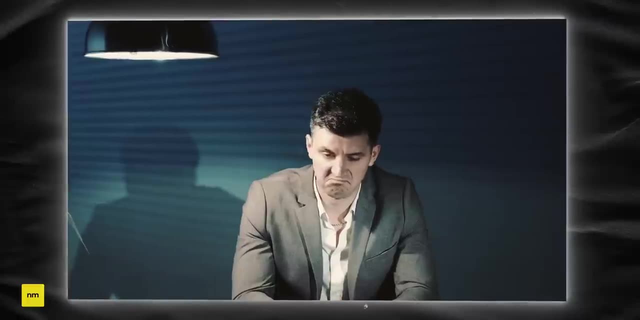 Now, while this could very well be 100 percent accurate, you can also see why investors took it so poorly: because it sounds like honey, I'm fine, or the little kid saying I didn't do it, or the suspect saying I can't remember where I was that night. It just doesn't sound. 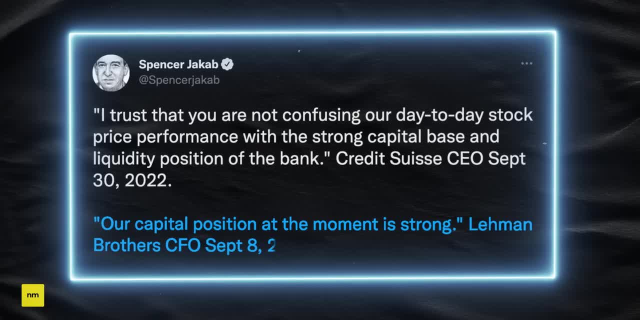 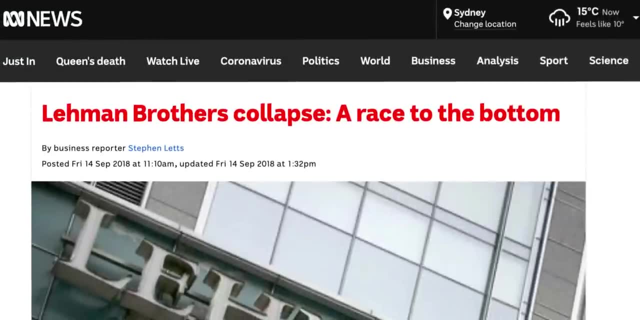 convincing, And I saw this tweet the other day. Apparently, the Lehman Brothers CFO said exactly the same thing as our good friend Ulrich back in 2008.. And we all know how that one played out. But just when it all sounded unconvincing, here's Credit Suisse stepping. 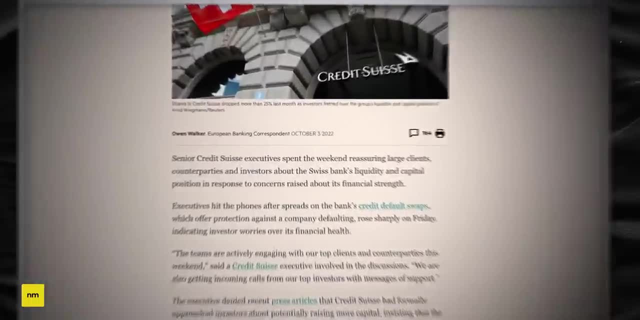 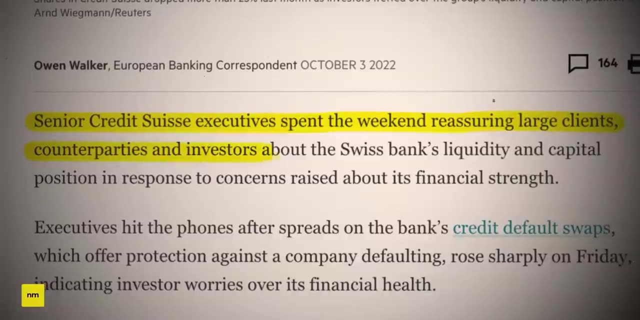 in it yet again. The most recent bit of news we've been seeing in this saga is the Financial Times reporting that quote: senior Credit Suisse executives spent the weekend reassuring large clients, counterparties and investors about the Swiss bank's liquidity and capital position. in response, 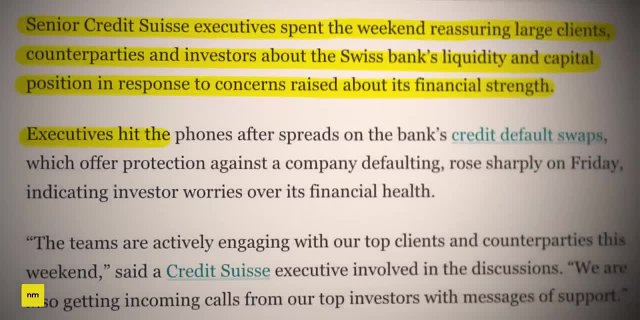 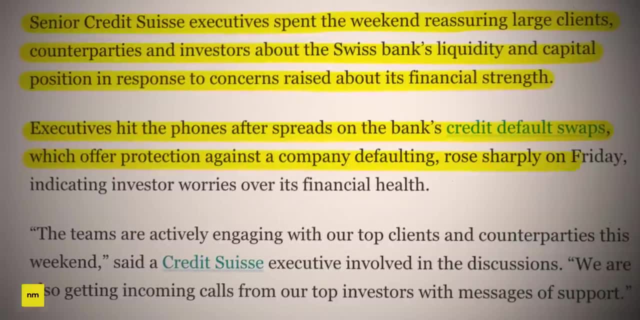 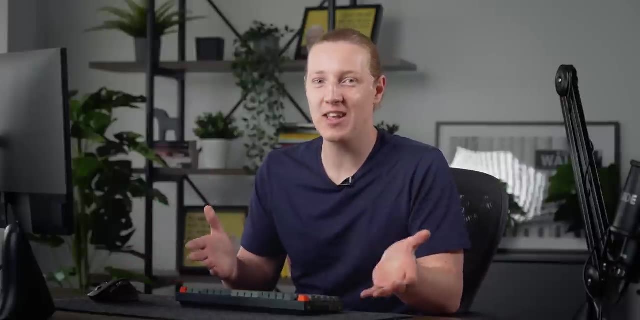 to concerns raised about its financial strength. Executives hit the phones after spreads on swaps, which offer protection against the company defaulting, rose sharply on Friday, indicating investor worries over its financial health. Again, this could all be 100 percent accurate, but it just doesn't really convince you. After: 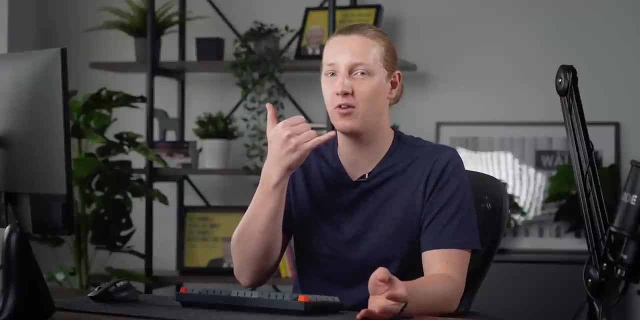 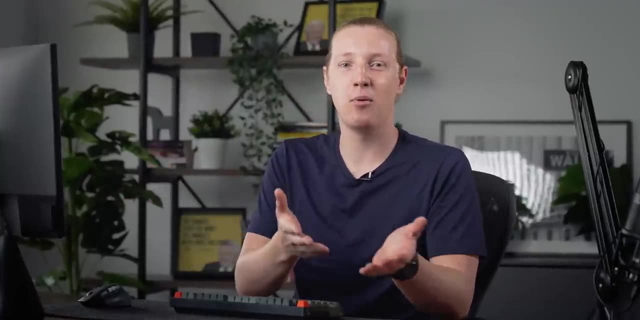 all, when was the last time you voluntarily picked up the phone and called your parents on a weekend just to tell them that nothing's wrong and everything's going to be all right? Exactly, And this is the main problem we're seeing now with Credit Suisse? They may be. 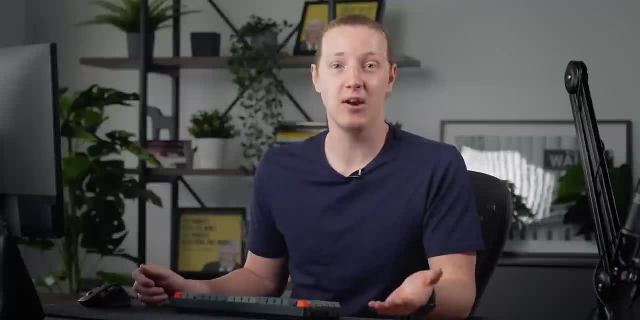 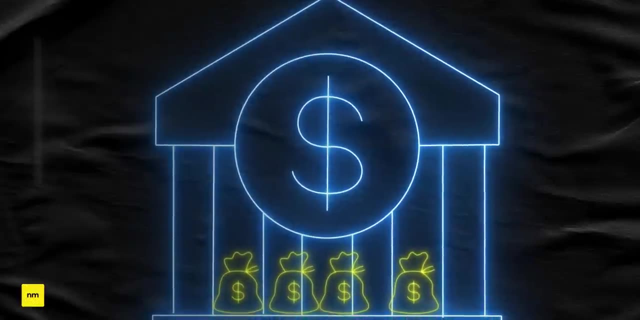 totally fine And in fact many financial institutions are even defending Credit Suisse. but the real problem here is there's a growing crisis of confidence And for a bank, a crisis of confidence can turn into a real financial crisis because clients can start to withdraw. 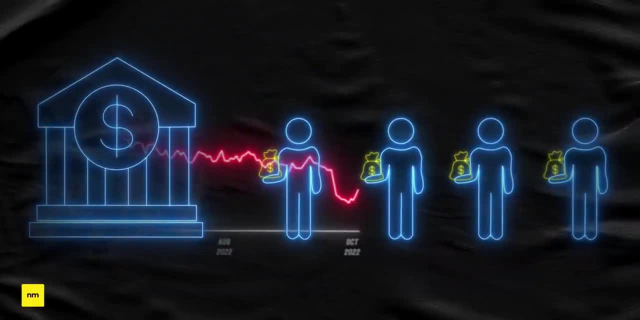 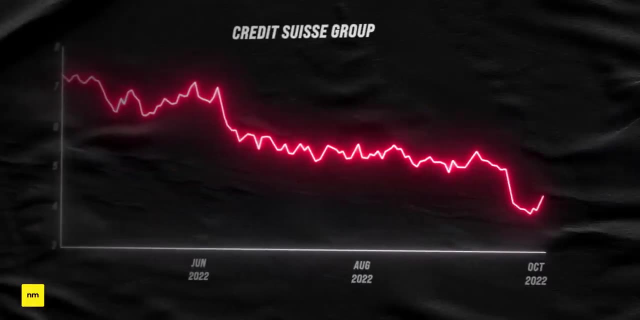 their money, And if enough people withdraw their money at the same time, then the bank can find itself in serious trouble. But here's the other thing: Even if it never gets to the point where there's a run on the bank, falling investor confidence could still spell big problems, Because- remember, Credit. 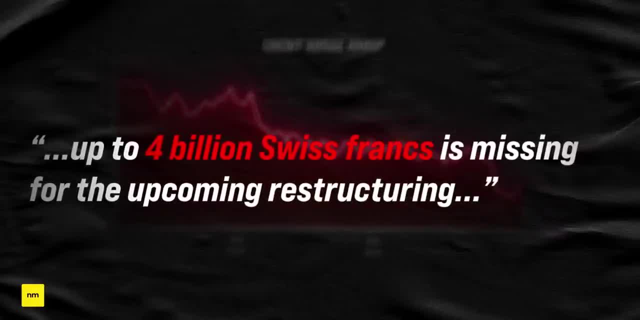 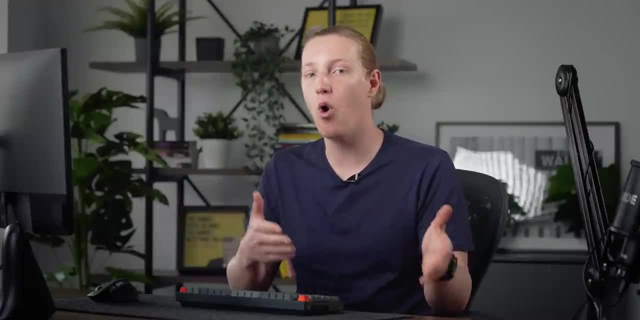 Suisse is supposedly trying to raise four billion Swiss francs to plug a hole. So every day that investor confidence declines and the share price falls, that looming task gets more painful. But that's really the story so far. A lot of people are shouting you. 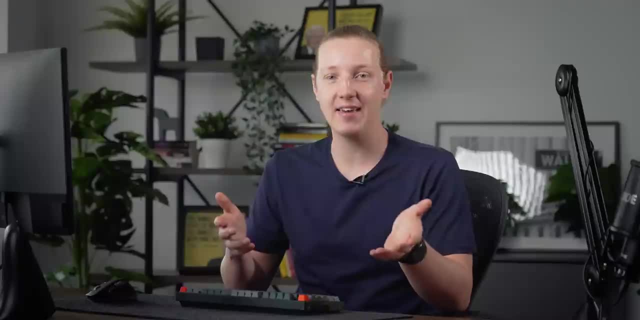 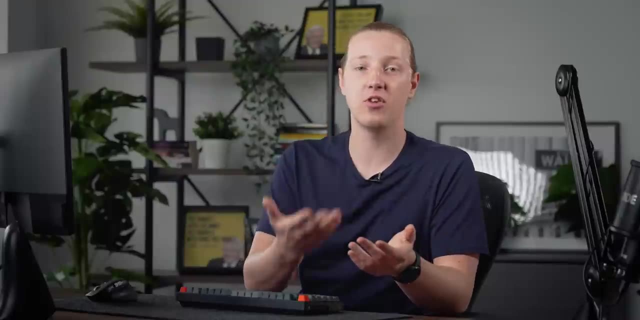 know Lehman moment on Twitter, But the truth is the bank just isn't very well managed and investors are losing a lot of confidence. And in the interest of fairness, I did want to show you guys the responses we've seen from those on the inside on Wall Street. The 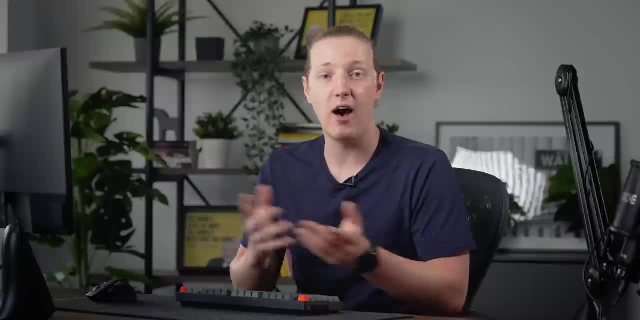 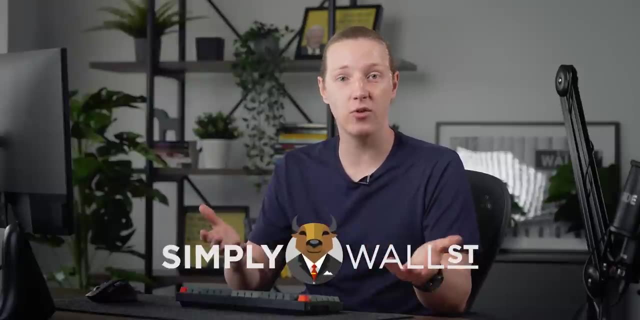 general consensus is that Credit Suisse is probably going to be okay. Now I would also encourage you guys to do your own due diligence on Credit Suisse before thinking about doing anything. For example, one analysis platform I like to use is simply Wall Street Full. 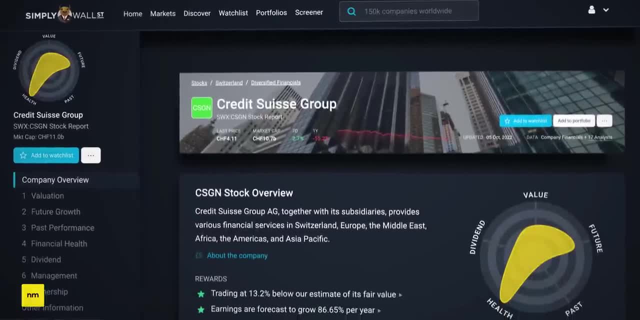 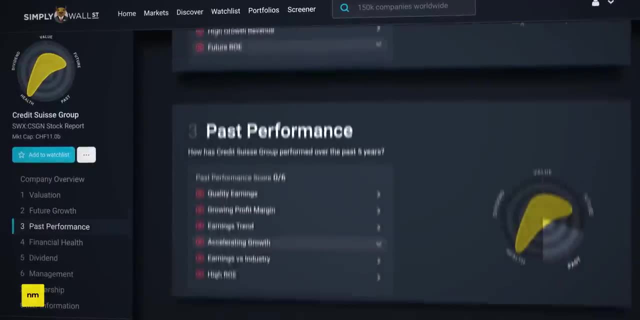 disclosure they are a channel sponsor, but I will leave their analysis of Credit Suisse down in the pinned comment. if you'd like to check that out further, You can explore valuation, future expectations, past performance and, importantly for this particular topic, financial. 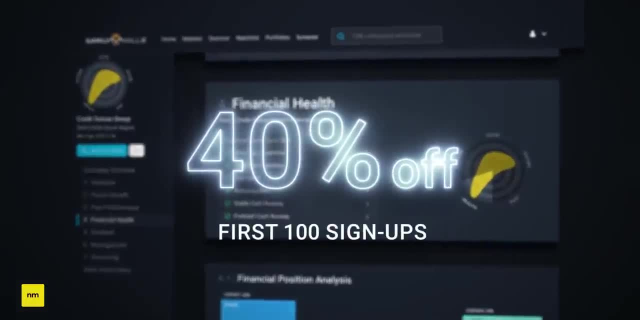 health. Also worth noting, you can get a sweet 40% discount for the first 100 signups through the referral link. So definitely check it out if you're interested. But with that said, here are a few examples of credit suisse. 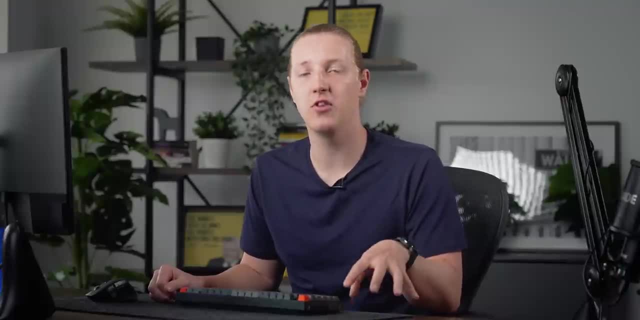 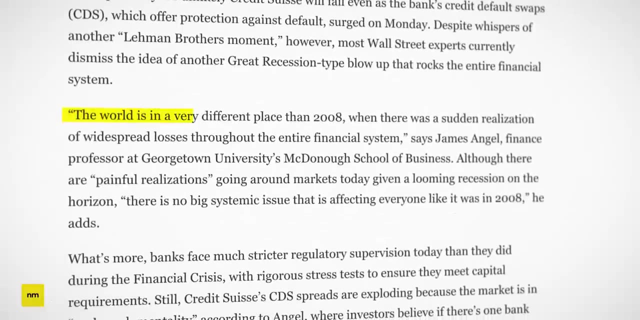 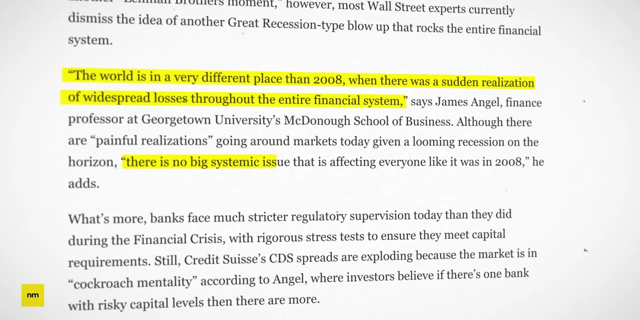 For example, a recent Forbes article quotes Georgetown finance professor James Angel, saying: quote: the world is in a very different place than 2008, when there was a sudden realization of widespread losses throughout the entire financial system. There is no big systemic issue that is affecting everyone like it was in 2008.. Vital Knowledge founder Adam Crisafulli. 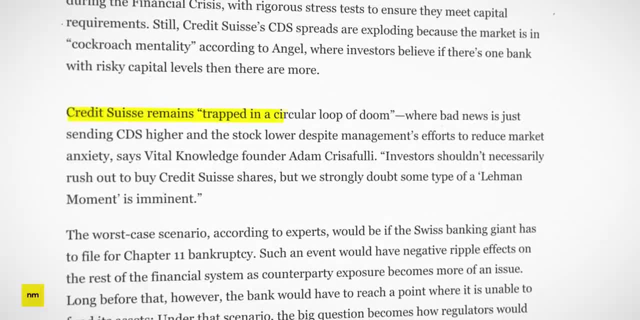 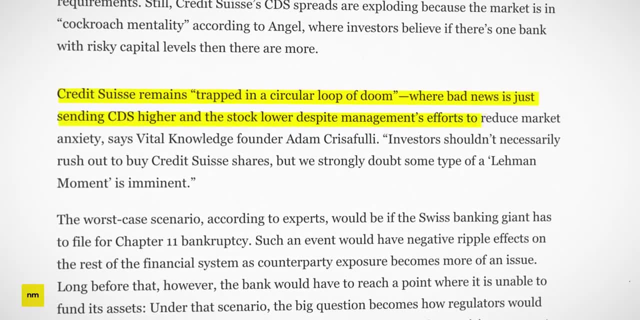 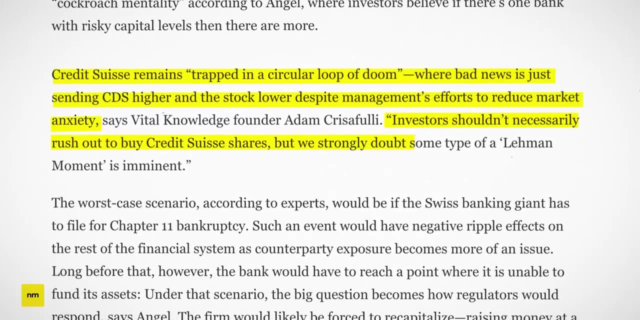 is also quoted saying that Credit Suisse simply remains trapped in a circular loop of doom where bad news is just sending credit defaults away. He says- quote: investors shouldn't necessarily rush out to buy Credit Suisse shares, but we strongly doubt some type of Lehman moment is imminent. City analyst Andrew Coombs said. 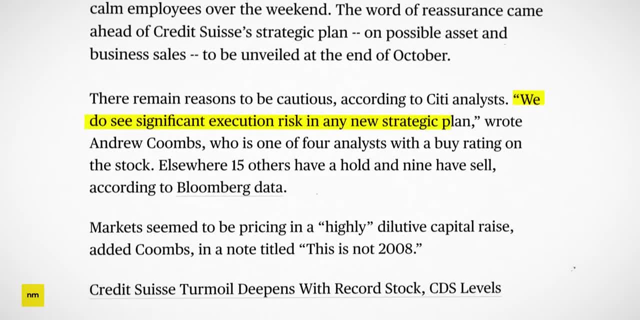 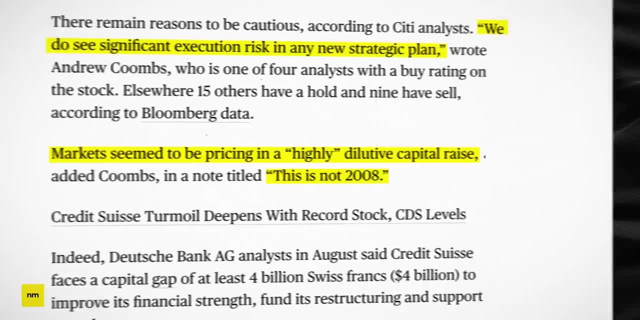 quote: we do see significant execution risk in any new strategic plan and the markets seem to be pricing in a highly dilutive capital raise. But he added: this is not 2008.. City managing director Keith Horowitz also chimed in saying, quote: we understand the nature of the.